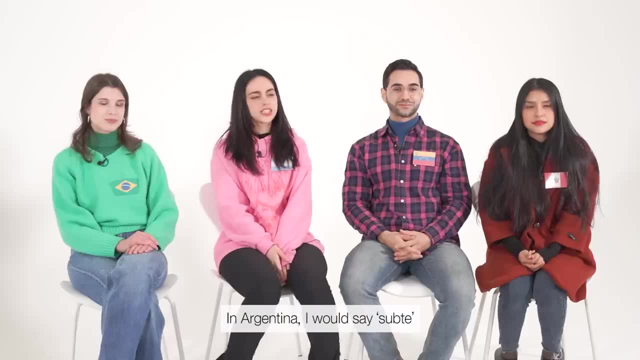 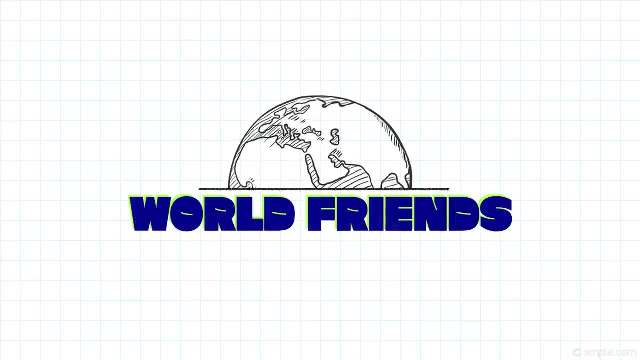 Horseshoe, Horseshoe, Horseshoe. In Argentina I would say supte Huh, Supte Soup, Like Supte. Hi, I'm Shannon. I'm from the United States. 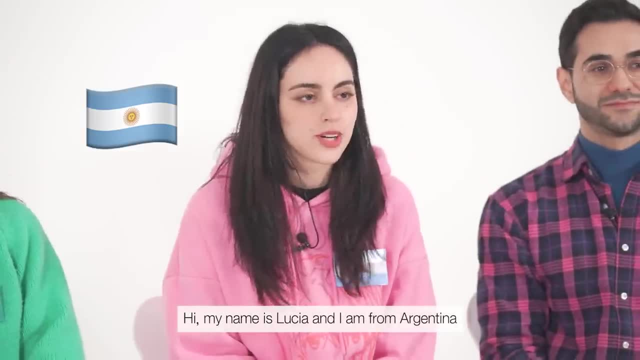 Hi, my name is Ana and I'm from Brazil. Hi, my name is Lucy and I'm from Argentina. Hello, my name is Antonio and I'm from Venezuela. Hello, my name is Damaris, I'm from Peru. 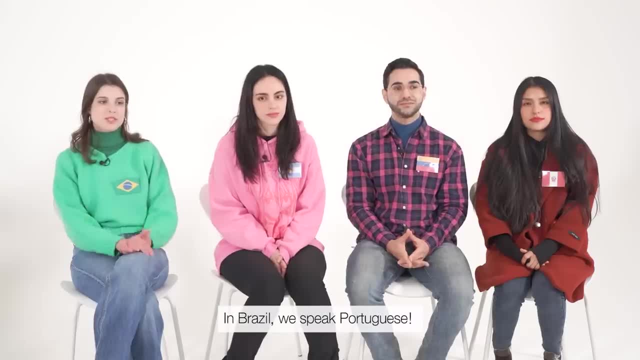 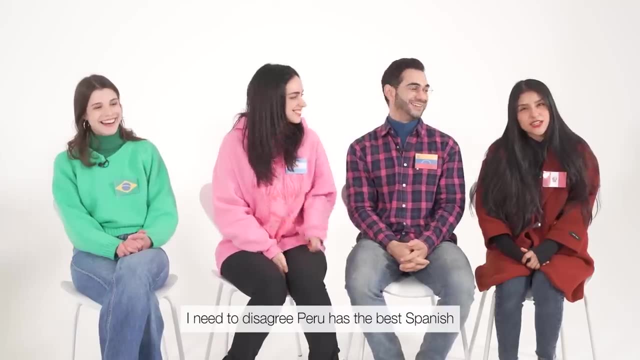 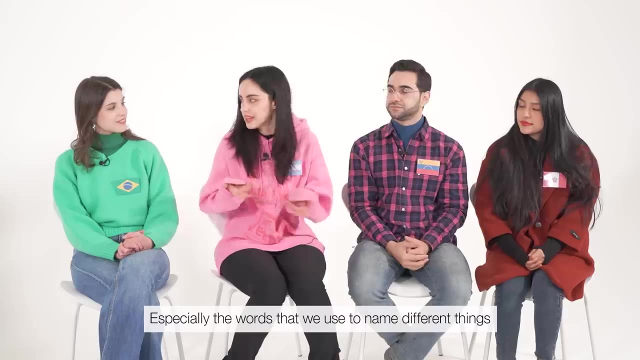 In the United States, we usually speak English. In Brazil, we speak Portuguese, We speak Spanish. We speak the best Spanish. in Venezuela, I need to disagree: Peru has the best Spanish. I think it would be pretty different, especially the words that we use to name different things. 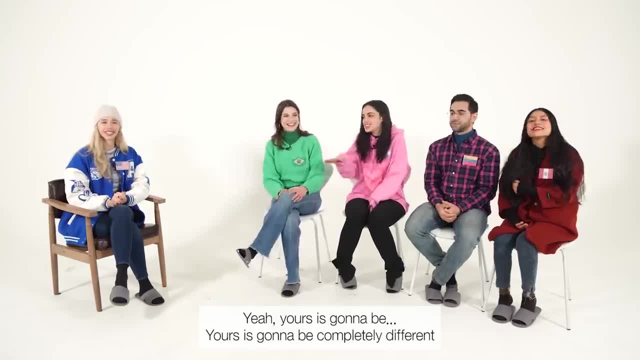 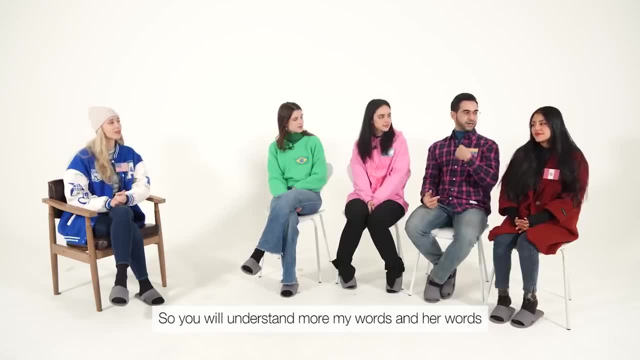 Yeah, mine is going to be different. Yours is going to be completely different. Yours is just another language, Mine is different. I think you are in the middle of us so you will understand more my words and her words. But we have like. 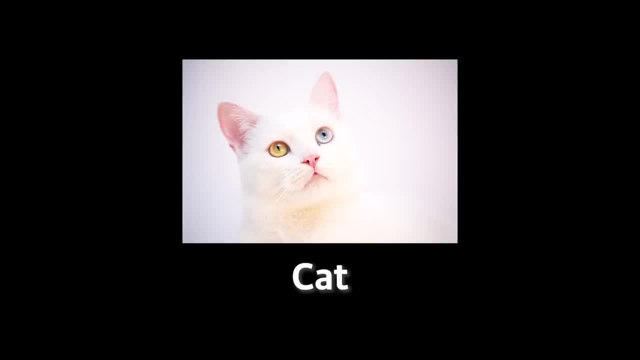 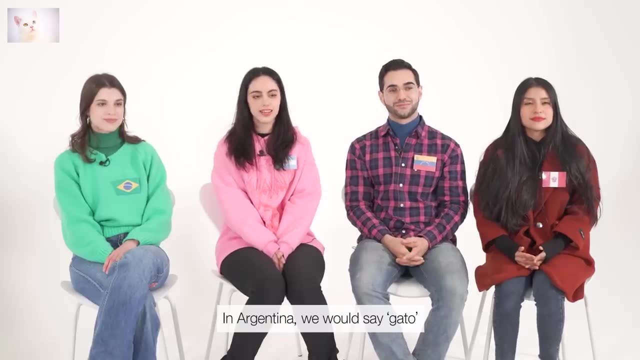 I think we might understand each other better. So in the United States we would say cat. In Brazil we would say gato. In Argentina we would say gato. In Venezuela we would say gato. In Peru we say gato. 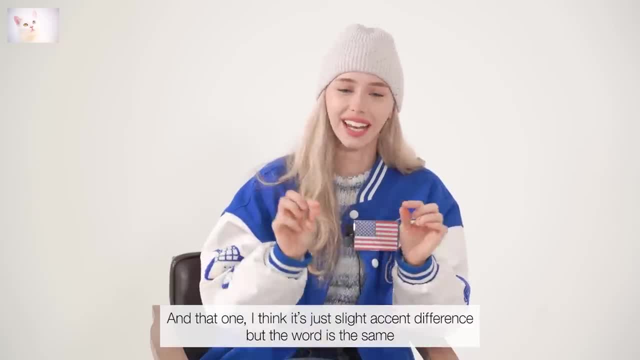 It's very similar. Yeah, it's too easy, And that one, I think, is just slight accent difference, but the word is the same. We will understand each other. Yeah, for sure. Gato, Gato, Gato. 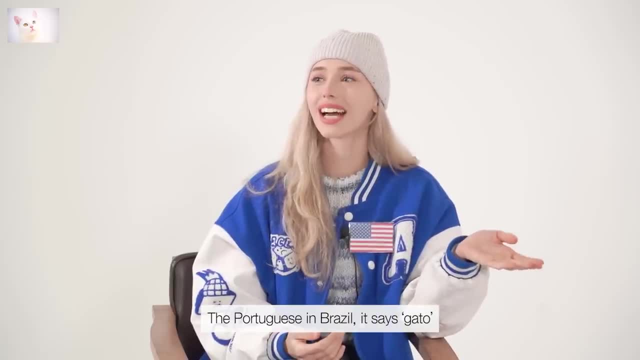 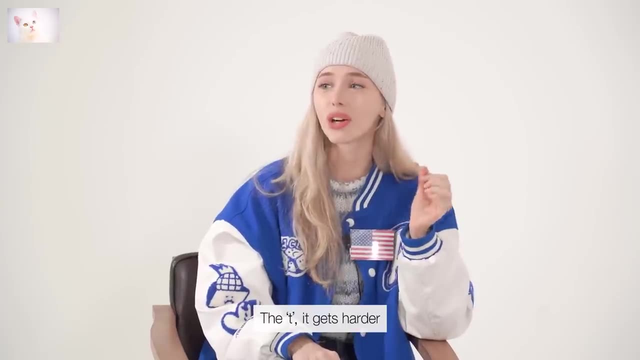 Gato, So the Portuguese. in Brazil it says gato. It's like gato. you know what I mean Like. the inflection is slightly different And then, as it goes across, the T gets harder with each one. 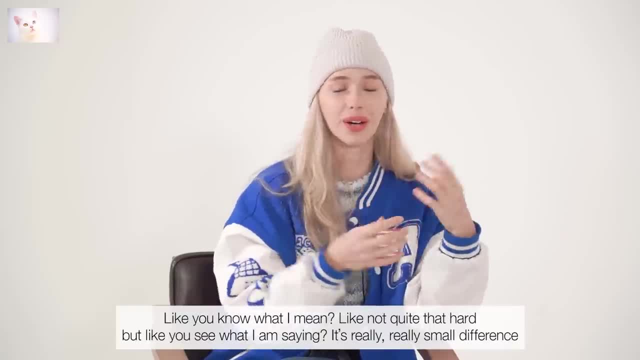 So like gato Gato, Like you know what I mean, Like not quite that hard, but like you see what I'm saying, It's really really small difference. So in the United States we would say red. 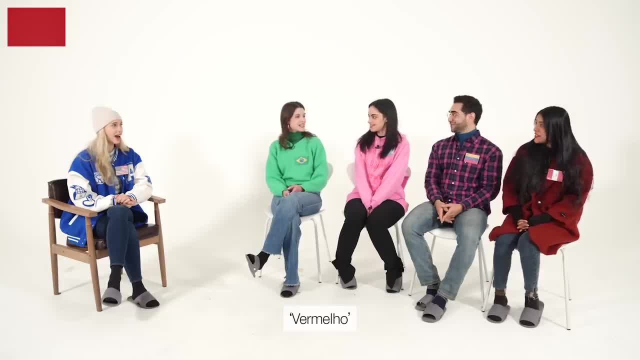 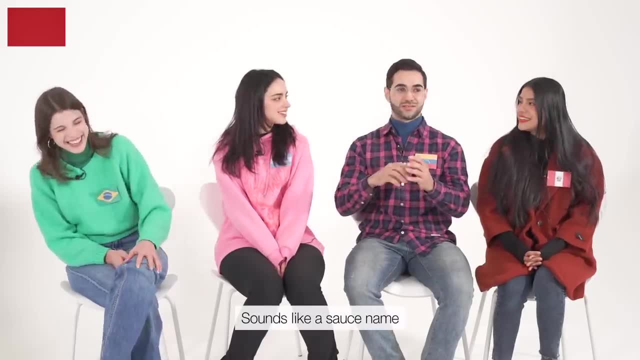 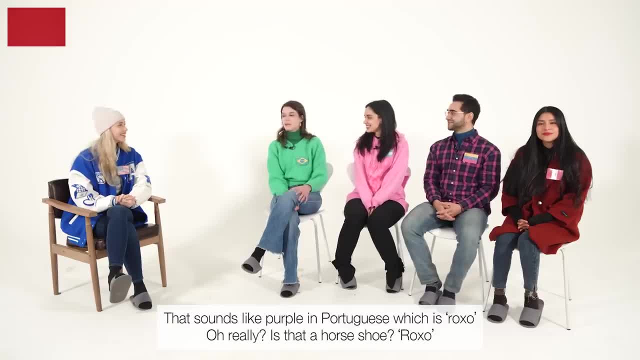 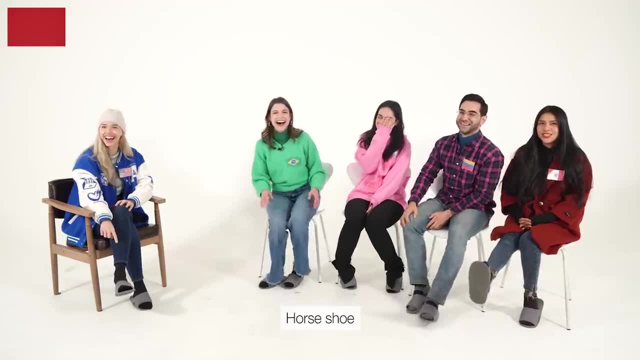 In Peru we say rojo. That sounds like purple in Portuguese, which is roxo Roxo. Oh really, Roxo, Roxo, Roxo, Oh shit, Yeah, definitely Portuguese is the weird one. I think we can all agree that that one. 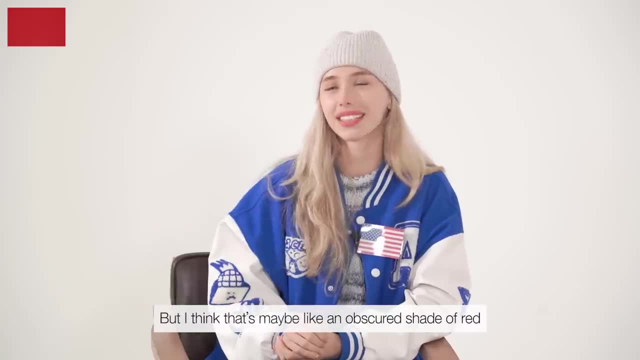 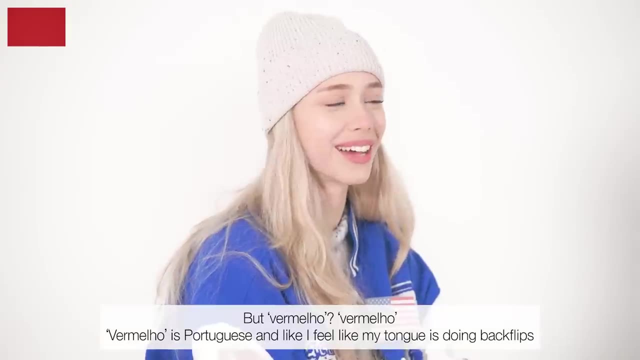 The word equivalent in English would say like vermilion, But I think that's maybe like an obscure shade of red. But vermelho Vermelho. Vermelho is Portuguese And like I feel like my tongue is doing backflips. 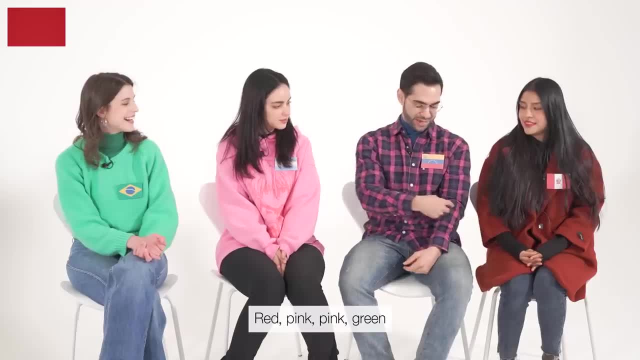 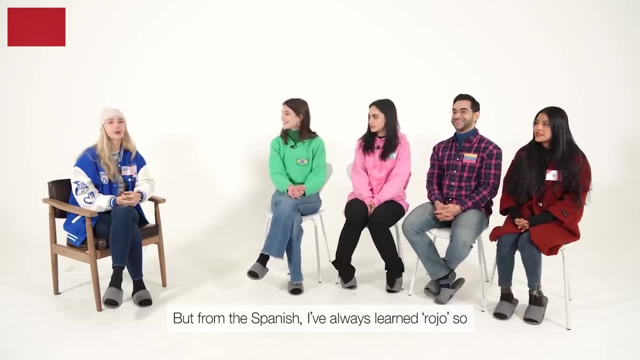 when I'm trying to speak Portuguese. Take a look here: Like Red, pink, pink, Green, Green- Yeah, That's Portuguese, But from the Spanish I've always learned rojo. So yeah, I can agree with you guys. 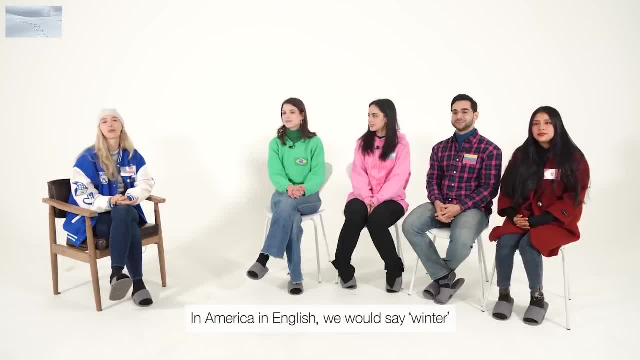 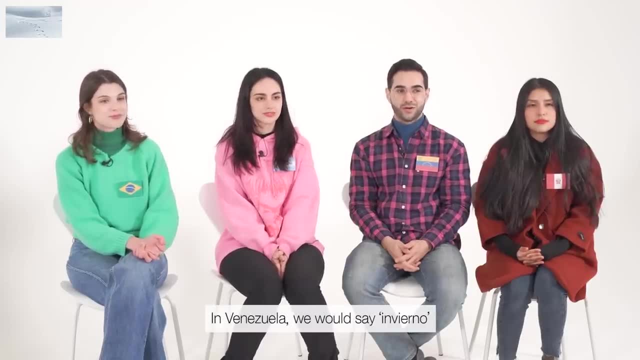 Yeah, In America in English we would say winter. In Brazil we would say inverno. In Argentina we would say invierno. In Venezuela we say invierno. In Peru we say invierno. 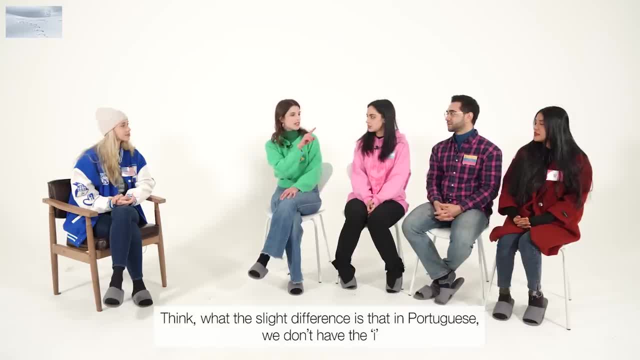 I think the slight difference is that in Portuguese, we don't have the I, You don't have the I. We would say inverno, Inverno. I did notice one small difference, though, between you two in the middle. 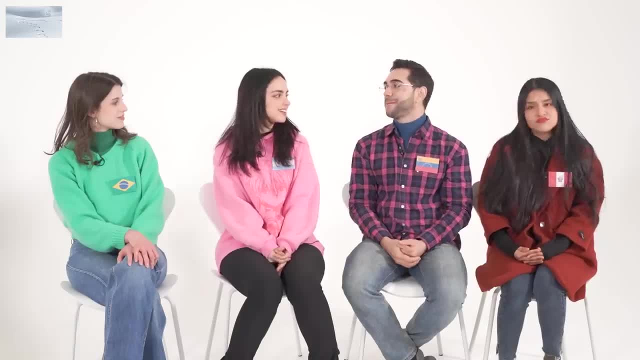 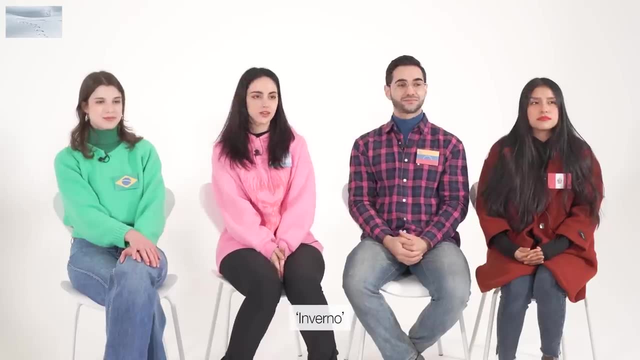 You had a harder V sound and his was B, Ah, B. Yeah, In Venezuela we don't say vi, We say vi. That was slight different. Inverno, Inverno, Inverno, Inverno. 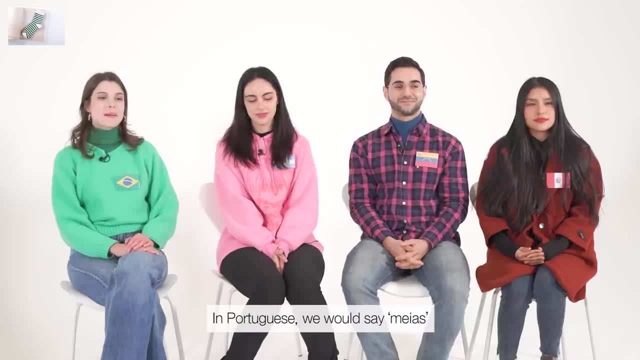 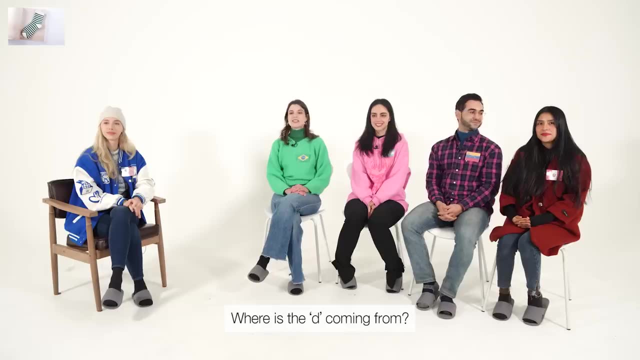 In English we would say socks. In Portuguese we would say meia. In Argentina, we would say medias. In Venezuela, we would say medias. In Peru we would say medias. Where's the D coming from? 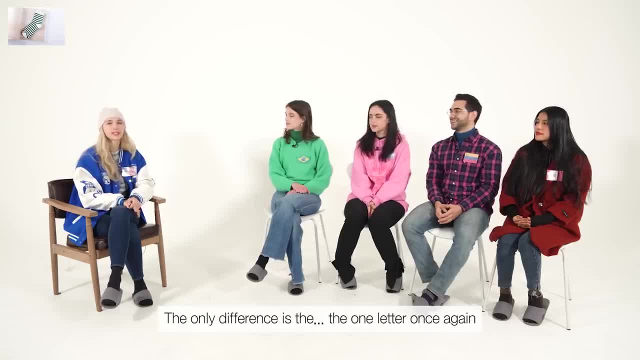 Medias? I don't know. Yes, Medias, Yeah, For me it pretty much sounded the same. The only difference is the one letter once again. So with invierno, the same word had one letter difference. Same thing for socks. 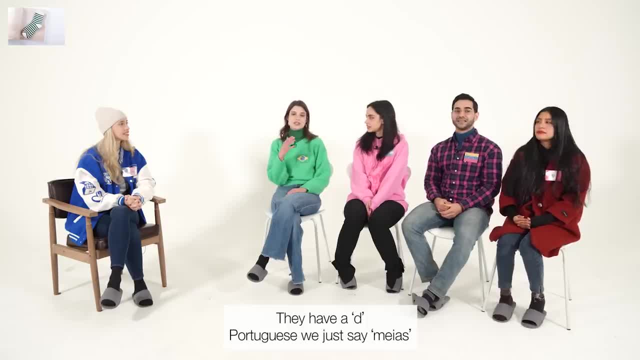 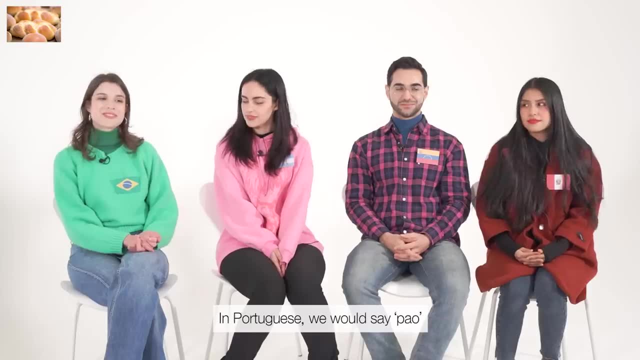 But the other three were relatively the same. Yeah, They have a D, Portuguese we just say medias. So no consonant there. No D In English we would say bread. In Portuguese we would say pão. In Argentina we would say pan. 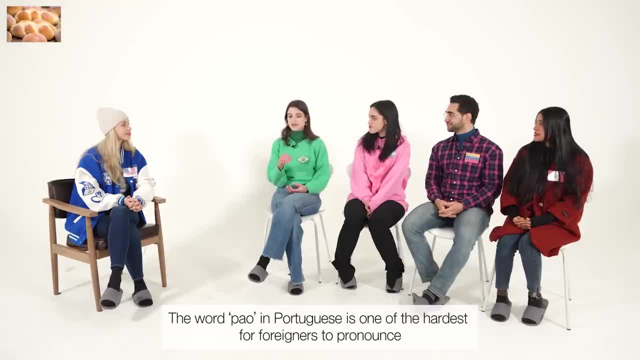 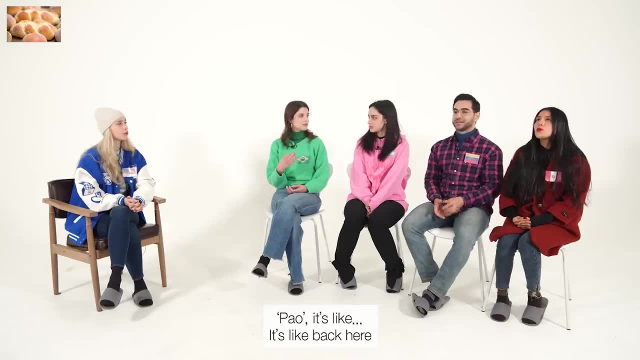 Marinarias. In Peru we say pão. The word pão in Portuguese is one of the hardest for foreigners to pronounce. Can you say it again: Pão, Pão, Pão, Pão, Pão. It's like. 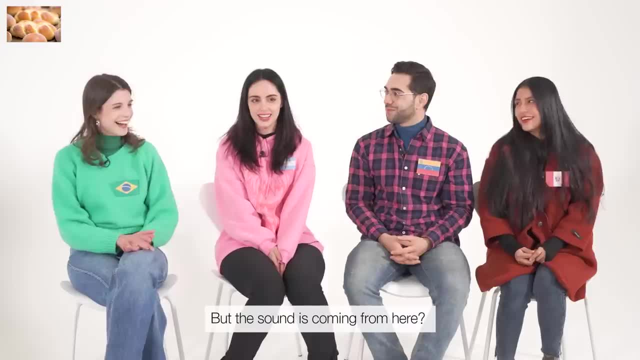 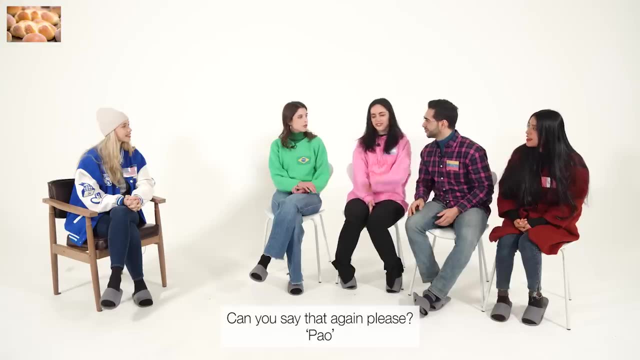 It's like back here, Pão. Pão Sounds like bone And the sound is coming from here. like Pão. It's back here, but like more on the top. Can you say that again, please, Pão. 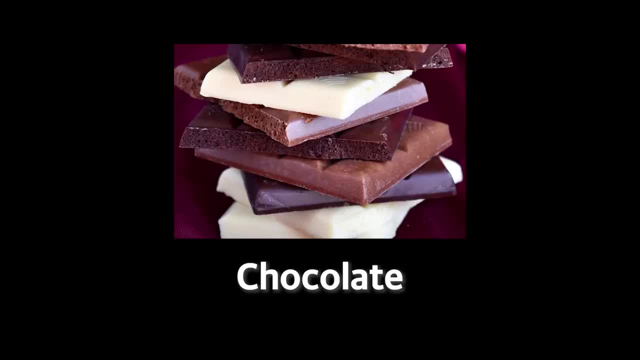 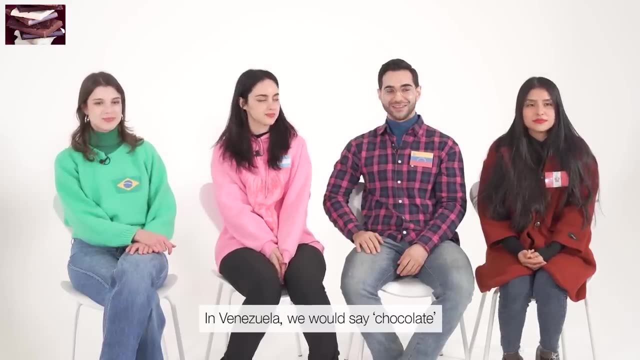 Pão, Pão. Next slide. So in English we would say chocolate. In Portuguese we would say chocolate In Argentina. we would say chocolate In Venezuela. we would say chocolate In Peru, we would say chocolate. Again, I'm in a different one. 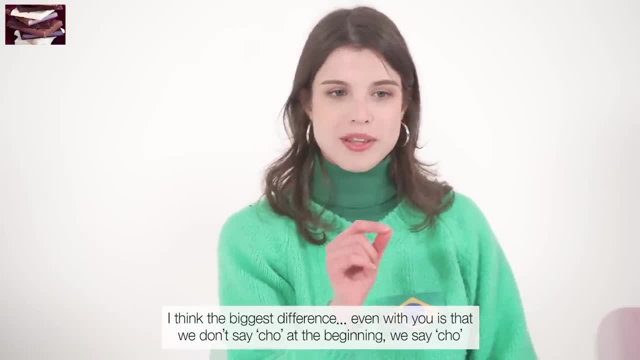 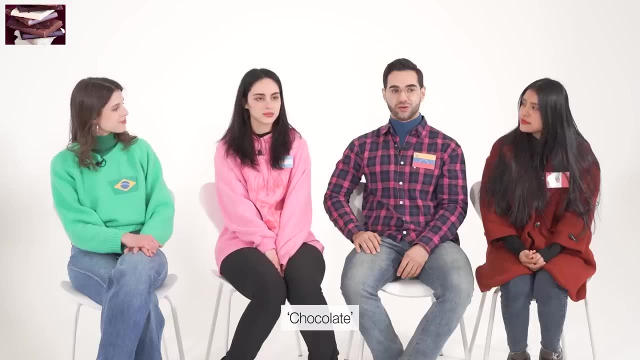 I think the biggest difference, even with you, is that we don't say cho at the beginning, we say sho, Mm, Chocolate And the T. then it's like chi sound, Chocolate, Chocolate, Chocolate. I think for this one, like in general the last three, their accent is the same, but 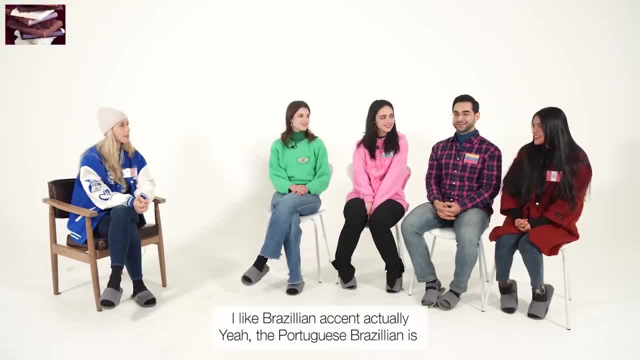 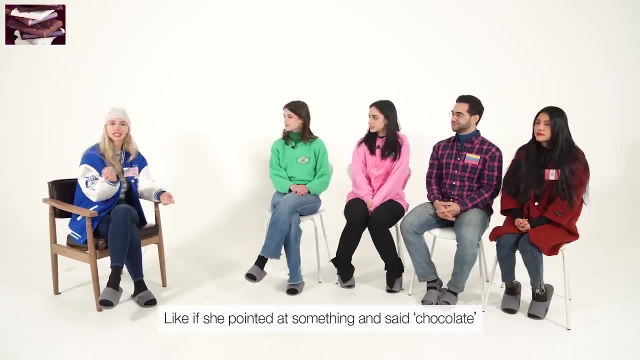 Chocolate, Chocolate. It's really different. I like the last dialect actually. Yeah, the Portuguese Brazilian is, But I do still think I could understand, Like if she pointed at something and said, oh, chocolate. like I could be like: oh, that's chocolate. 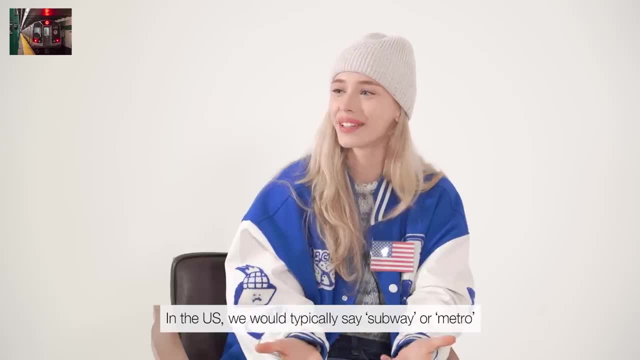 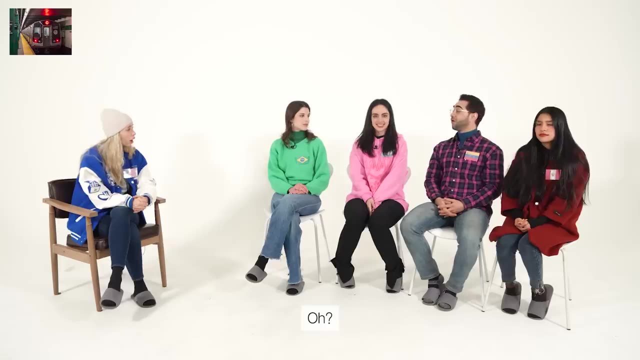 Like it makes sense. so In the US we would typically say subway or metro. In Portuguese we would say metro. In Argentina I would say subte, Oh, Subte, Subte. In Venezuela we say metro. 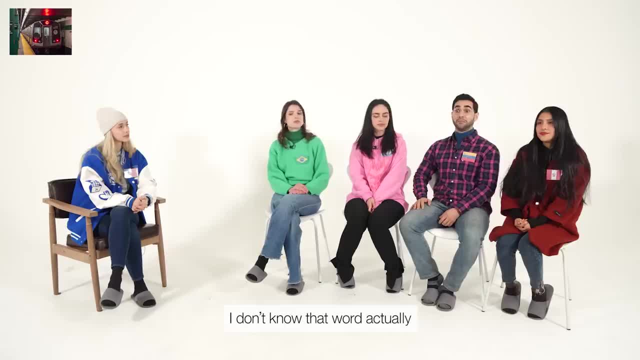 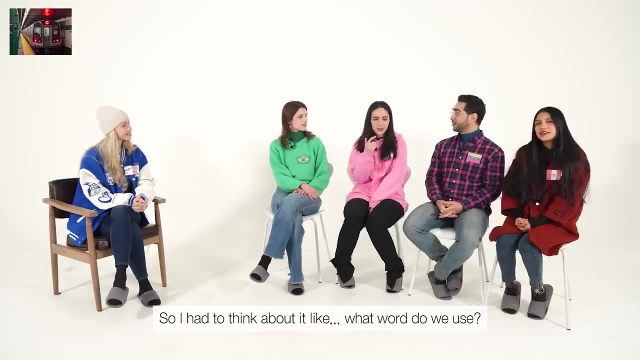 In Peru we say metro or metropolitana, Mm. I don't know that word. actually In my city we don't have subways, Mm. So I had to think about it like what word do we use? 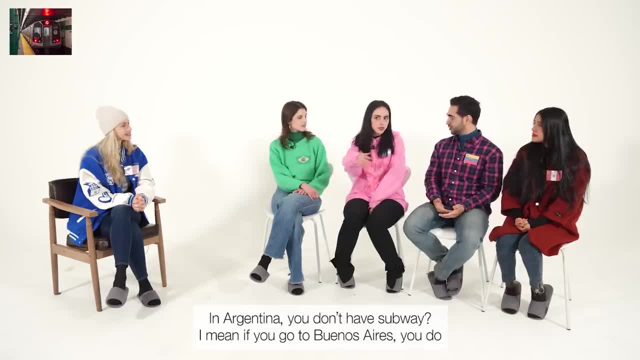 Yeah, Oh, really Yeah, I don't have a subway In Argentina. you don't have a subway. I mean, if you go to Buenos Aires you do, Ah, okay, okay, But But it's outside, right. 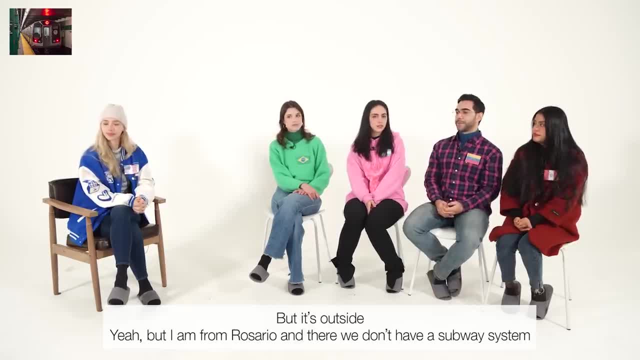 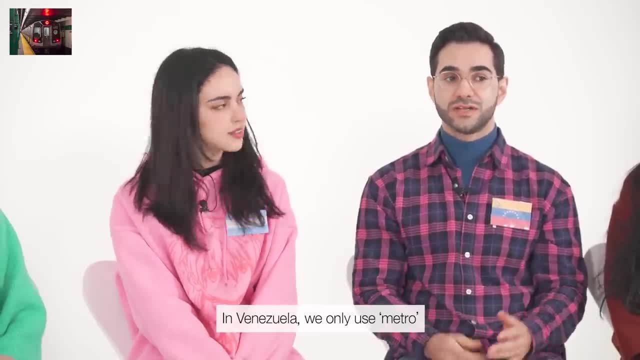 Yeah, but I'm from Rosario and there we don't have a subway system, So I had to think about it. but I'm pretty sure we would say subte. I never heard anybody say metro Mm. In Venezuela we only use metro. 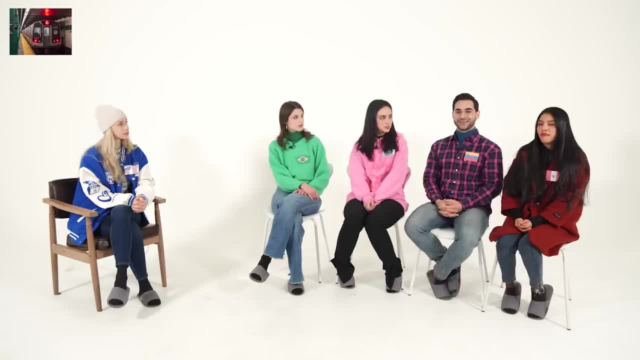 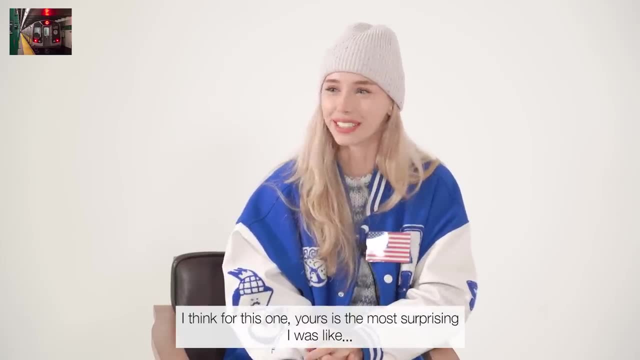 We don't use metropolit, or subte, Subte, Subte, Subte- Those are foreigner words for me, Mm. I think for this one yours was the most surprising. I was like soup, Soup. 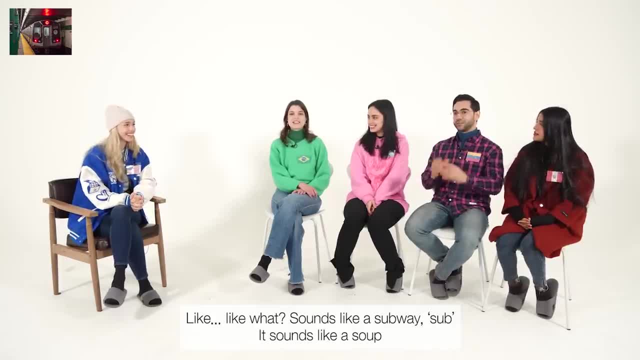 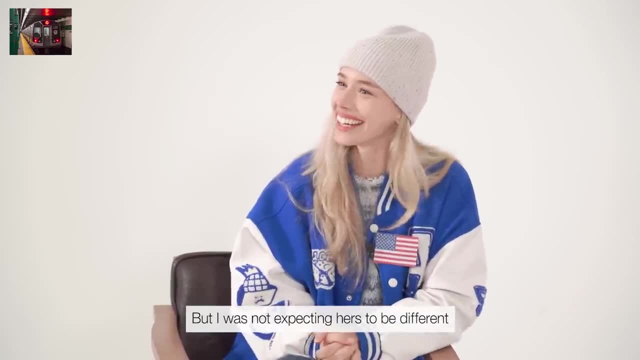 Subte, Like, Subte Like. It sounds like a subway, just something. It sounds like a soup. So that one was. I was expecting the Portuguese to be different, but I was not expecting her to be different. In America we would say computer. 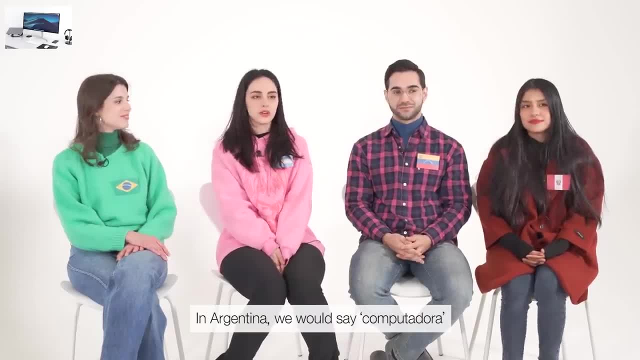 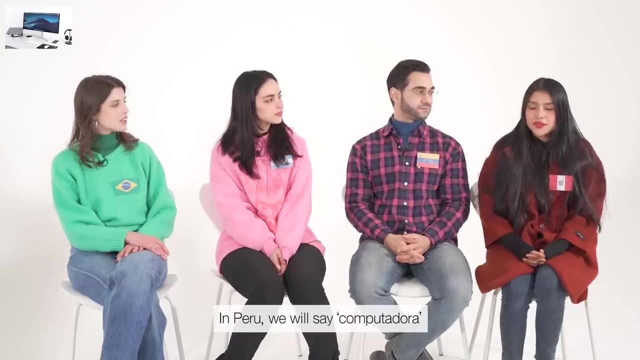 In Portuguese we say computador And in Argentina we say computadora. Okay, in Venezuela we have two words. We say computadora o ordenador. In Peru we say computadora o ordenador. Si, What about if it was like a laptop? 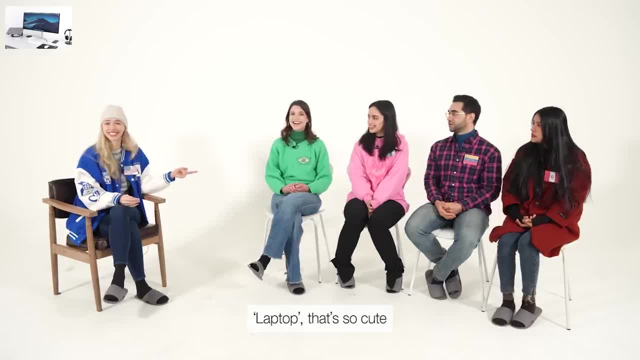 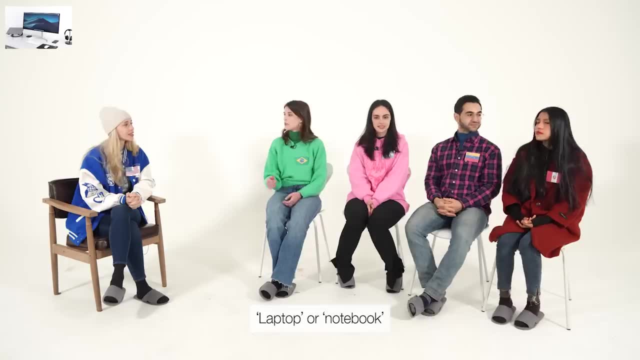 Would you guys say laptop, Laptopi, Laptopi. That's so cute. We would just say notebook, Notebook. Oh okay, We say both laptop or notebook, Laptopi or notebooki, Notebooki. It sounds like notebooki. 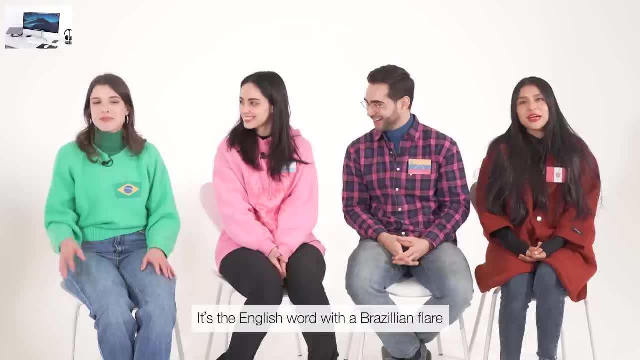 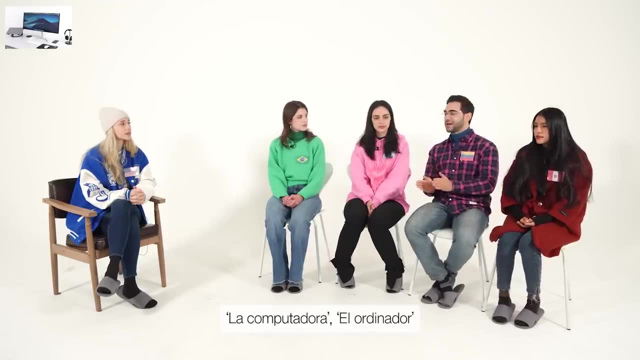 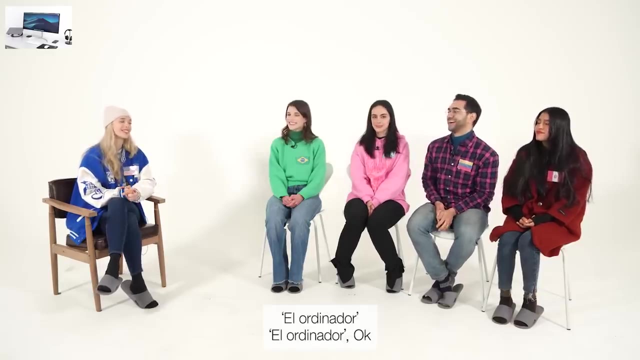 These sound like fake words. It's the. you know, it's the English word with the Brazilian flair. Yeah, Yeah, Portuguese is. It's cute, It's adorable. La computadora el ordenador. Okay, that's a lot of R's. 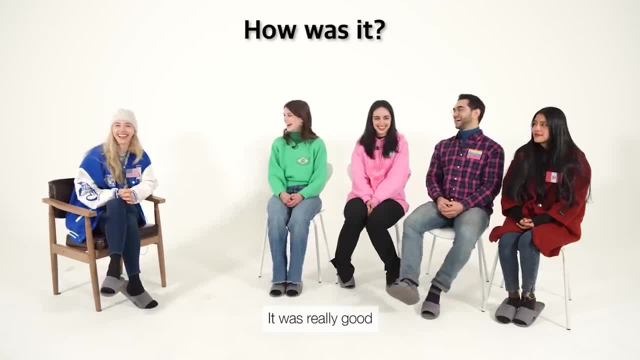 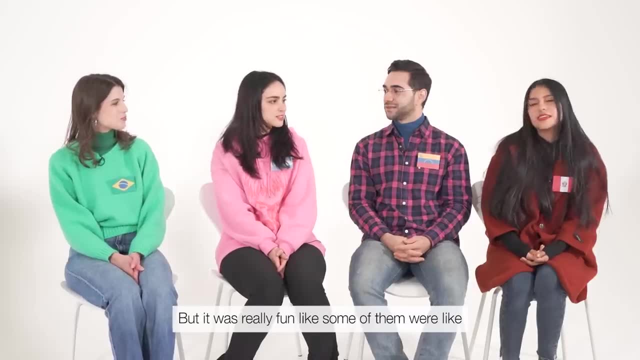 Very nice, very good, It was really good. Yeah, it was fun, I thought. I mean I guess the words are kind of similar to Spanish, But it was really fun. Like some of them were like new for you. 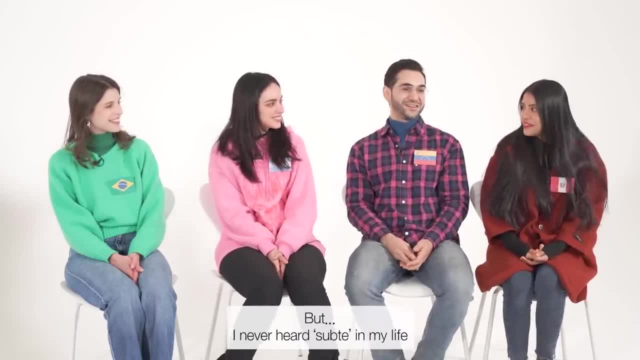 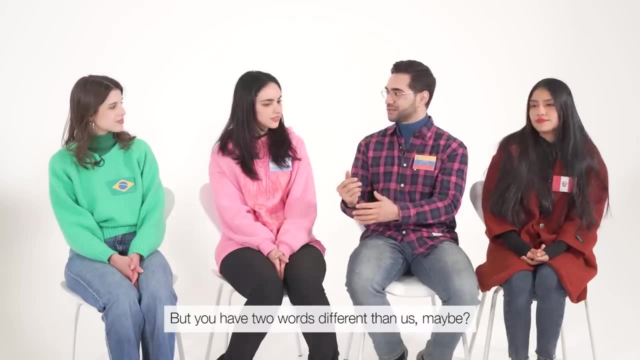 Subte. I knew for her Subte. It was the first time in my life, Really. Yeah, me too First time. I think the Spanish is pretty same, But you have two words different than us, maybe Subte. 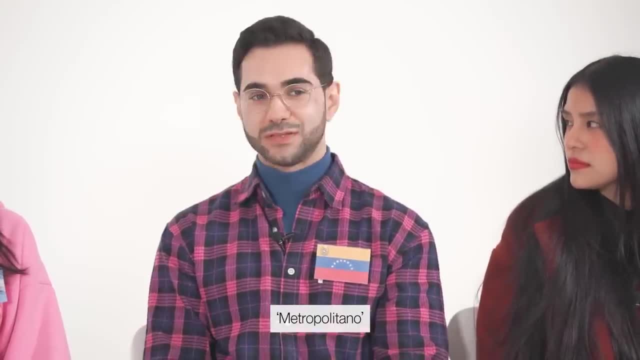 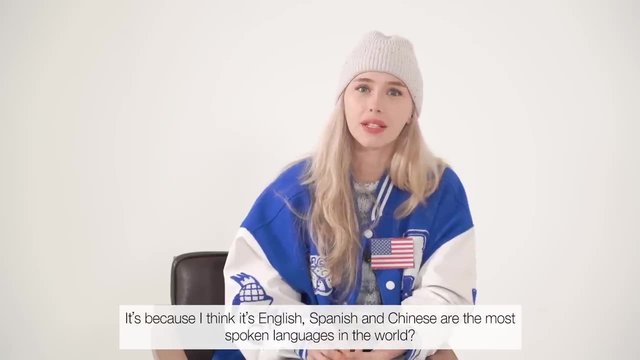 And? And what was the other one, Notebook? Ah, notebook, Metropolitano. You two have two different words: Subte, Yeah, I think that's. what's really cool about it, though, is because I think it's English, Spanish. 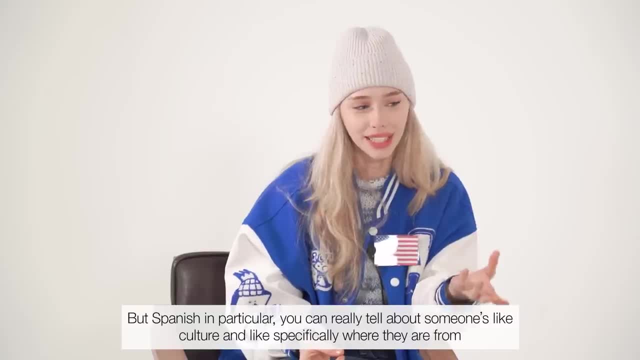 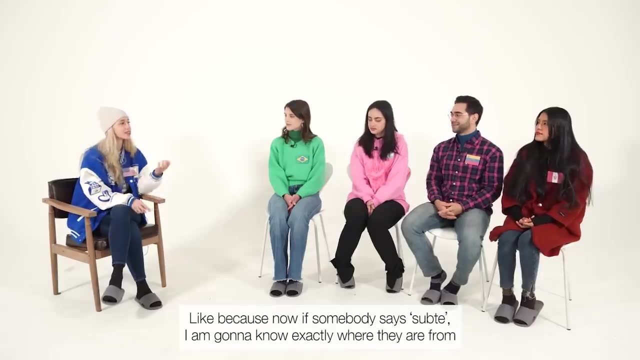 and Chinese are the most spoken languages in the world. Yes, But Spanish in particular. you can really tell about someone's like, culture and like specifically where they're from, based on those tiny differences, Right Like, because now if somebody says Subte, I'm gonna know exactly where they're from. 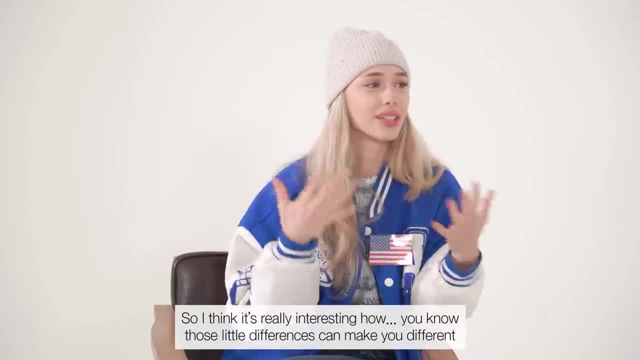 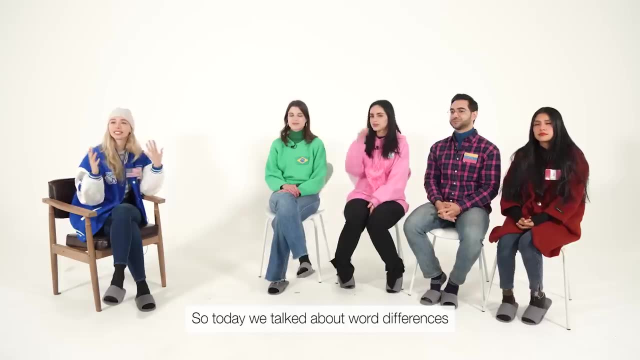 But other Spanish speakers might have no idea. so I think it's really interesting how you know those little differences can make you different, but everyone still speaks Spanish. There's still a Spanish world. Yeah, We understand each other. Yeah,